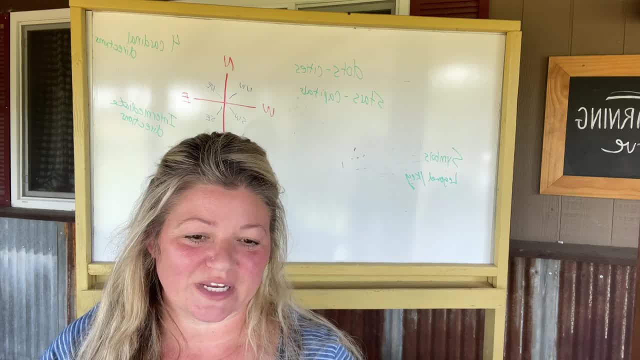 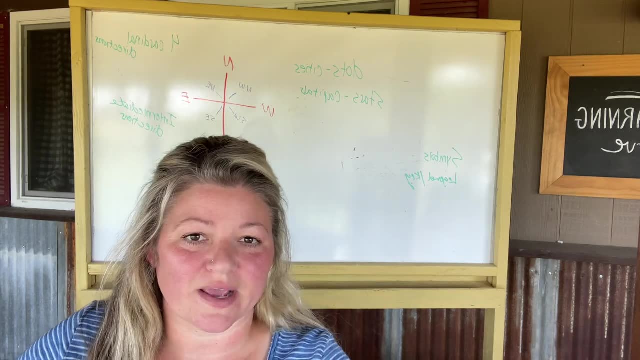 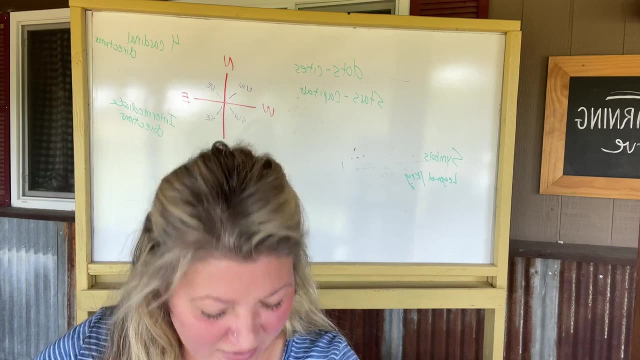 fun to do for the kids, and so I created a worksheet. It's a map. I will go ahead and link that in the description box for you guys as well. I went to the dollar tree and I got several pieces of the foam board and painted what looks to be done by a kindergartner. I'm a little embarrassed. 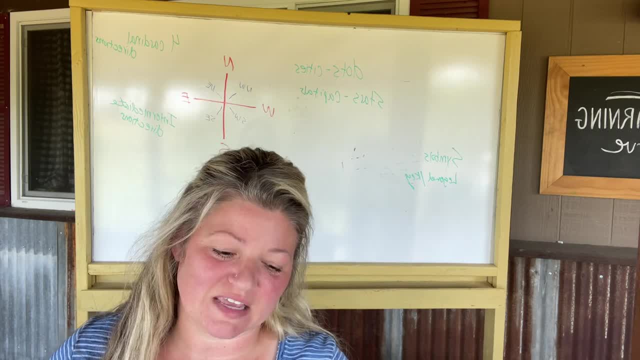 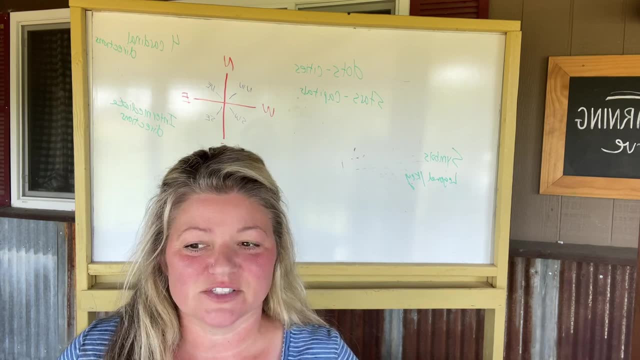 to show you guys, but I painted these large symbols that would be found on a map, on my map that I created, and so I'm going to put them out in the field and I'm going to give the kids instructions and also a compass, because we are 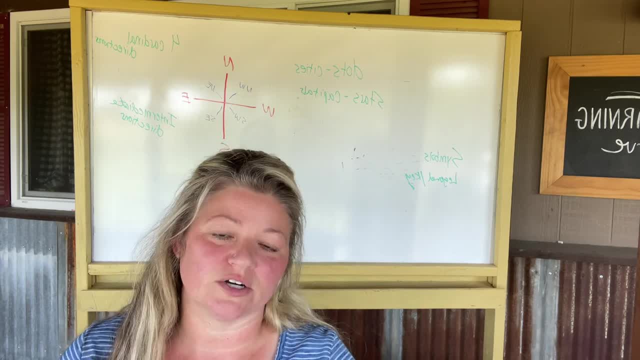 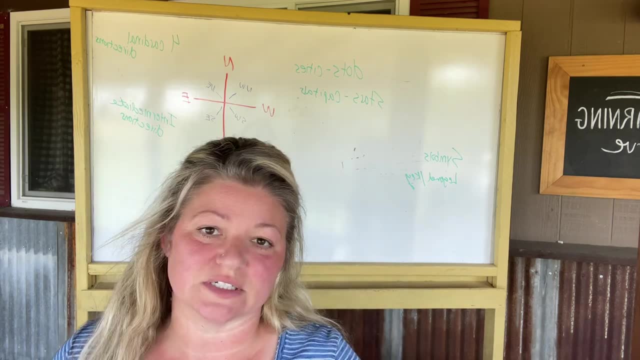 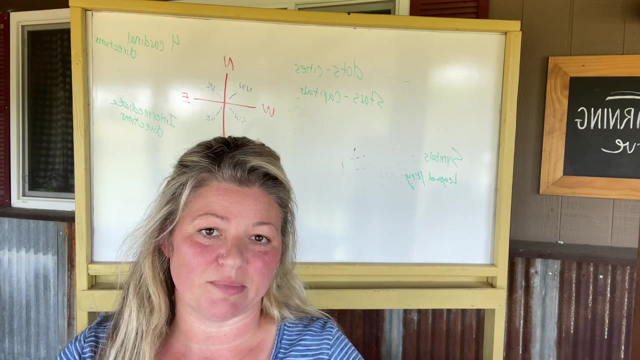 discussing the four cardinal directions as well as the intermediate directions. So they're going to be learning how to follow the instructions that I give them, and it will take them to various places in the yard, to the different symbols that I put out, and then they might just find a tree. there It is. 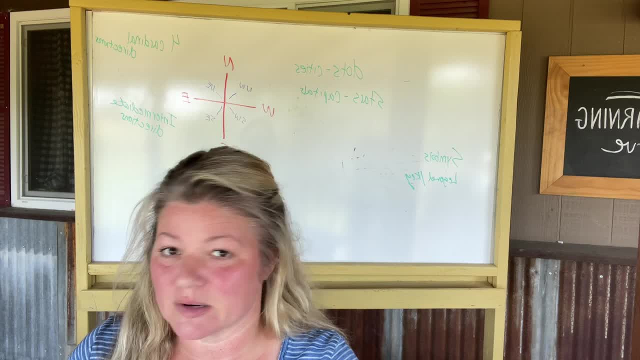 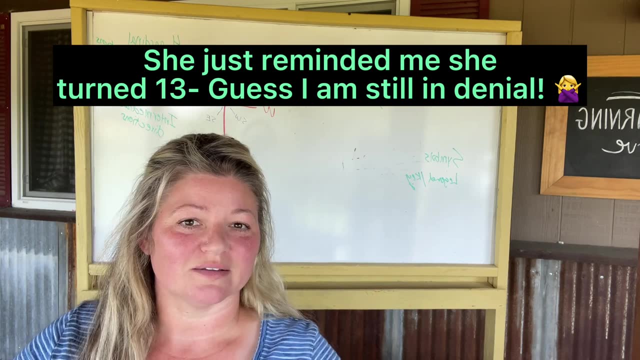 a little windy outside and my husband said: I don't think that you're going to be able to do it. the poster boards are going to fly away, but we are going to try. My 12 year old was asking me why? why do we need to learn how to read a map when we have GPS? Well, I reminded her that a zoo. 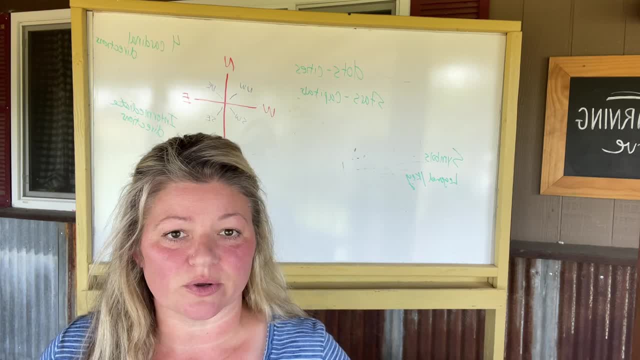 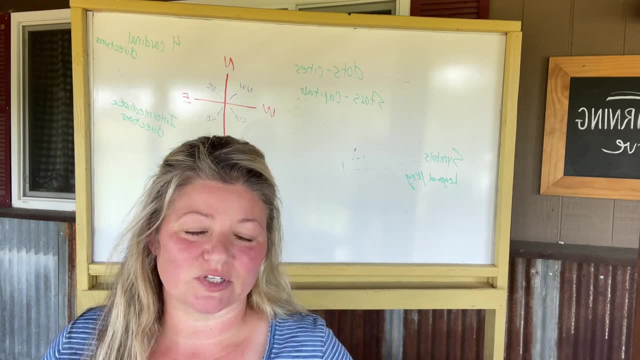 amusement parks, all these places that we like to go to. they're all giving out a guide at the entrance to show you where to go, and so those are maps. so it's important to learn how to read a map, and it's also important because they're related to me. 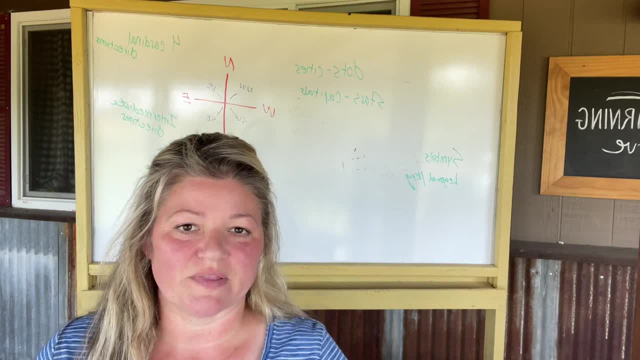 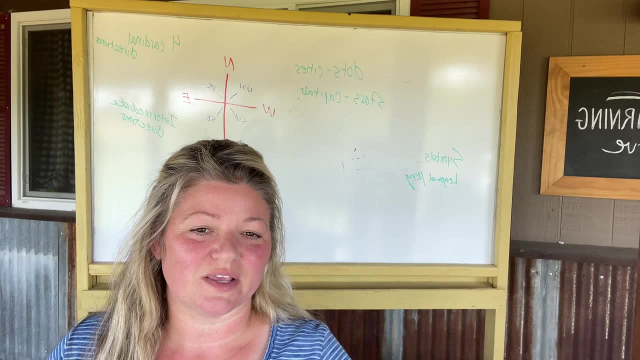 and I have a horrible sense of direction. heaven forbid that gets passed down to them. they need to be prepared, so we are going to go ahead and get set up and we will see you out in the field. okay, so I've given the kids their instructions. and Paisley, do you have your compass? 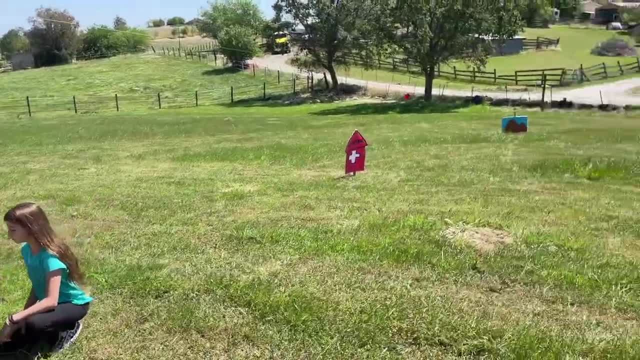 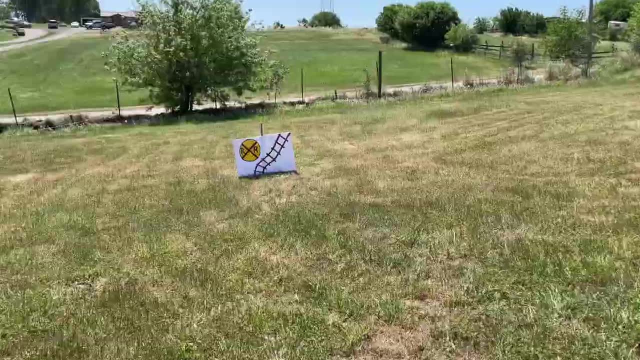 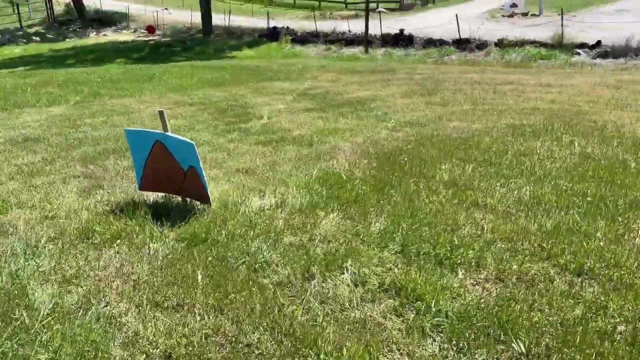 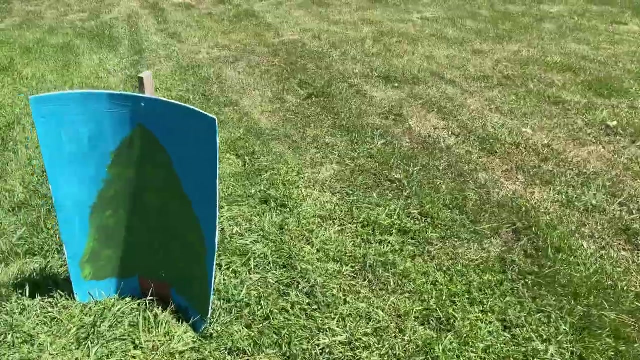 yeah, okay, so we have a compass and, as you can see, we've set up different symbols for the kids out here: campsites, we have the railroad, have the ocean- it is really windy out here- and then we have the mountains, we have the hospital and we have a forest. 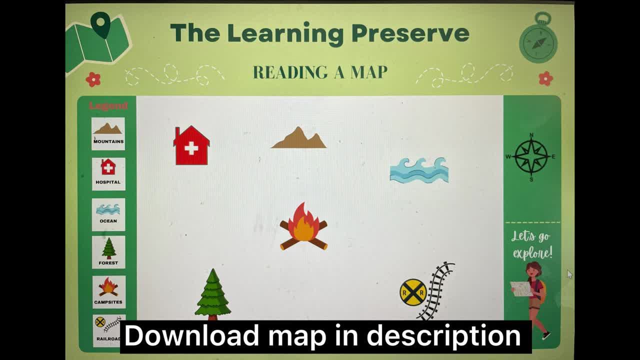 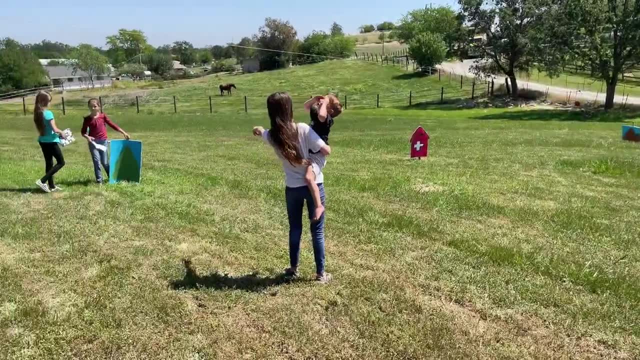 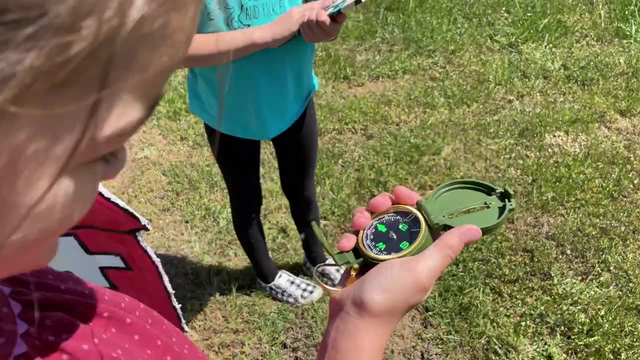 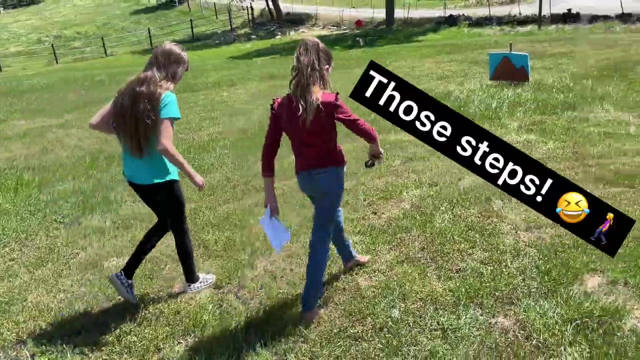 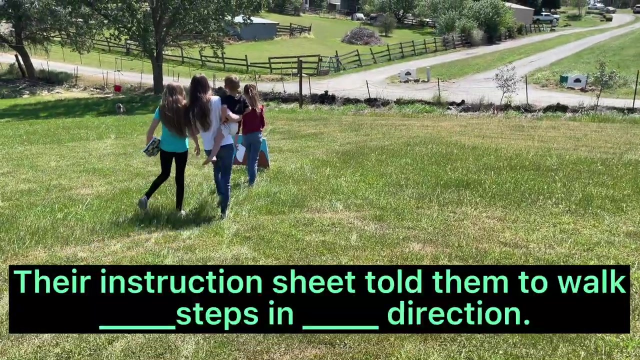 life is a winding road, no telling where it goes, driving through days and nights, won't stop for traffic lights. and I, I really want to know, really want to know. if I I'll never figure out where the road goes, if I, even if I'm falling down, I will keep on searching for my 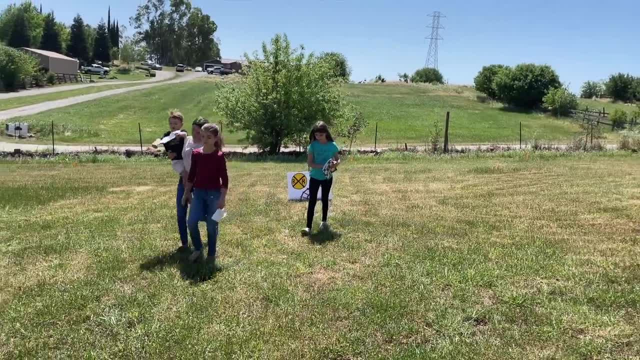 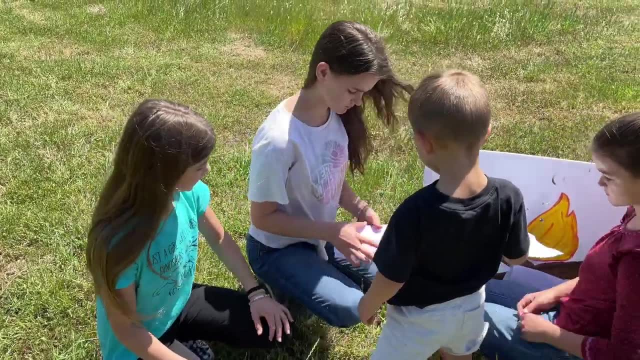 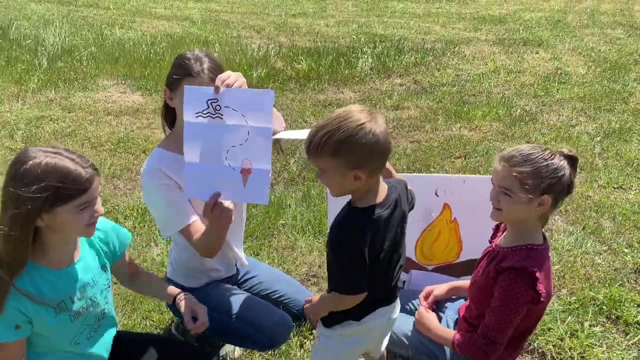 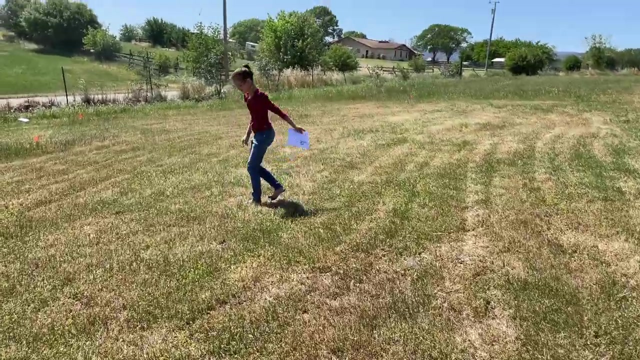 eyes, you can say: I lost my mind. I will keep on holding my hand, swimming and ice cream. oh, you like swimming? uh-huh, daddy was right. I hate it when daddy's right. it is like a dream. It's too windy up here. Okay, thanks. 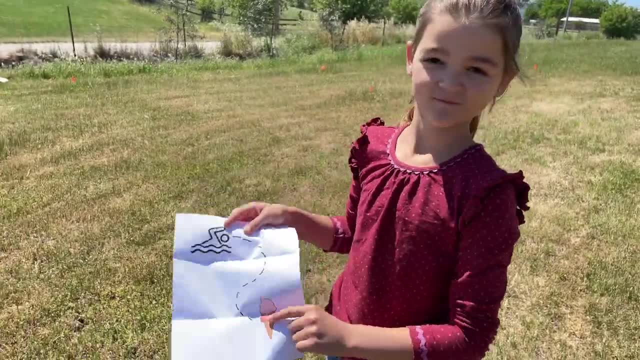 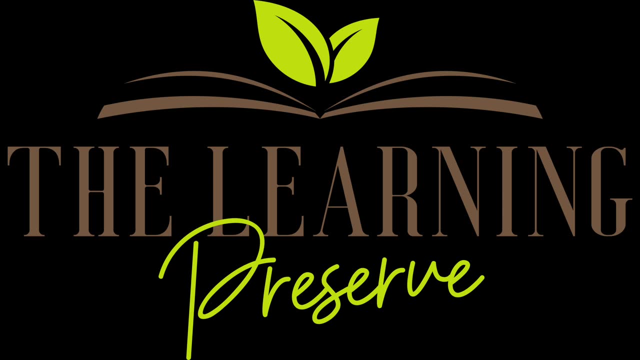 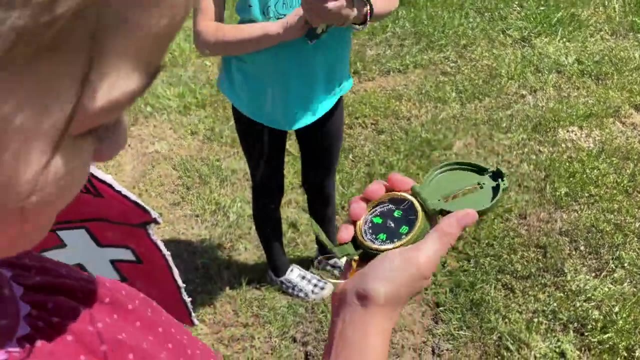 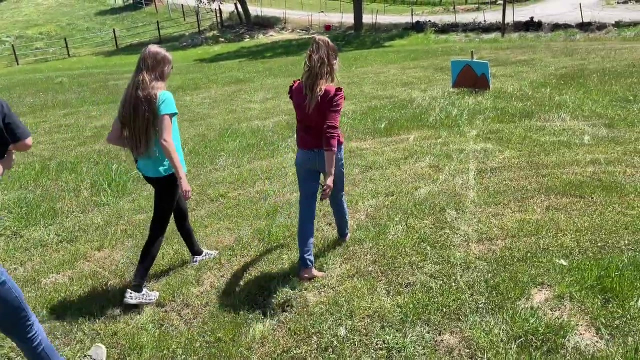 Well, we get to go swimming and get ice cream. Thank you so much for watching our video. Bye. If I never figure out where the road goes, even if I'm falling down, I will keep on searching for my highs. Thank you. 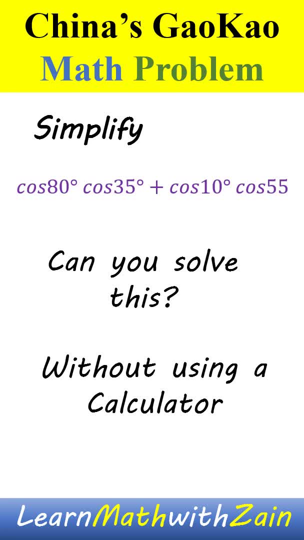 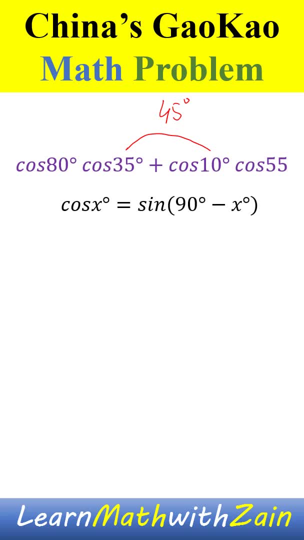 Can you solve this without using a calculator? Let's begin to solve it. 35 degree plus 10 degree is 45 degree. We know that cos x is equal to sine 90 minus x degree. Using this, we can write cos 80. 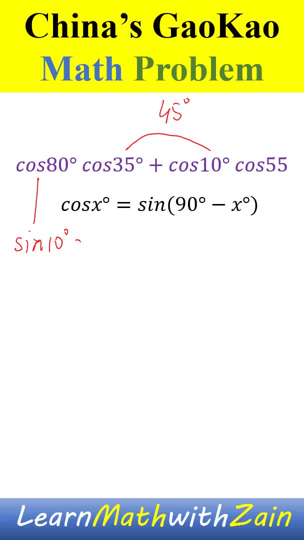 is sine 10 degree into cos 35 degree plus cos 10 degree and cos 55 is sine 35 degree. Now, using this identity, we can write: this is sine 10 degree plus 35 degree, This is equal to sine 45 degree and sine 45 degree is equal to 1 over square root of 2, and this is the.